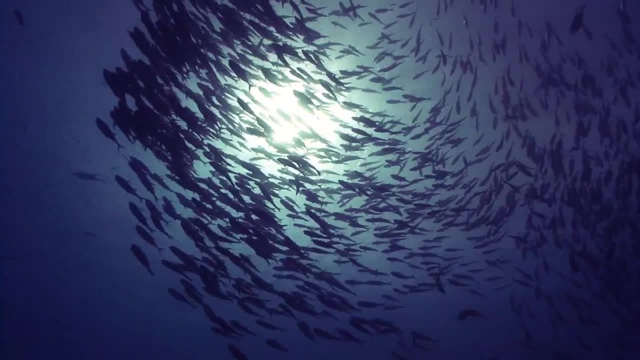 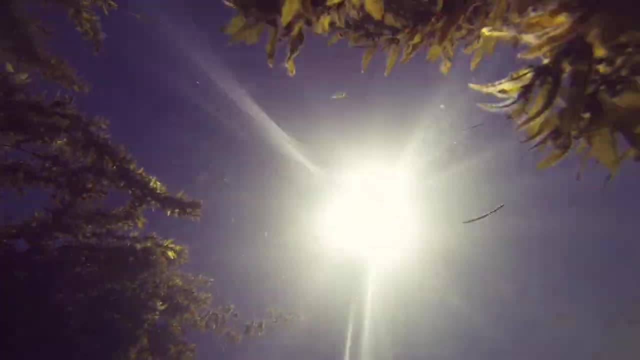 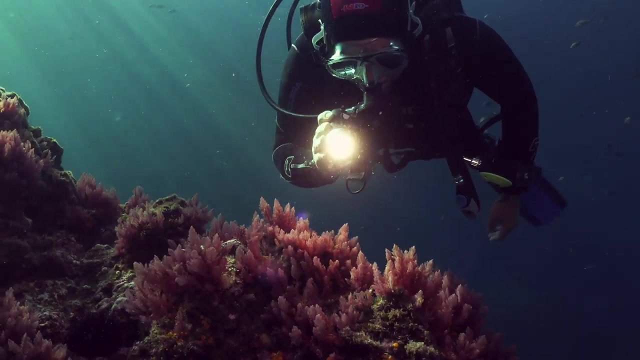 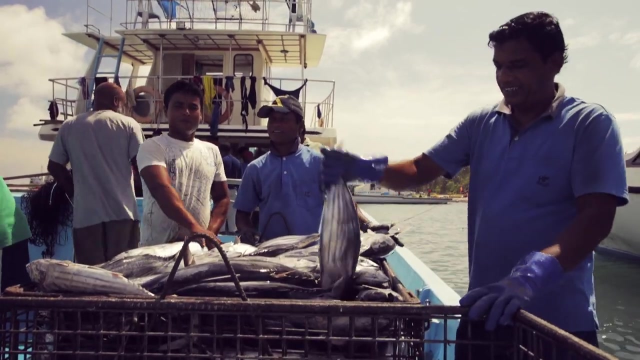 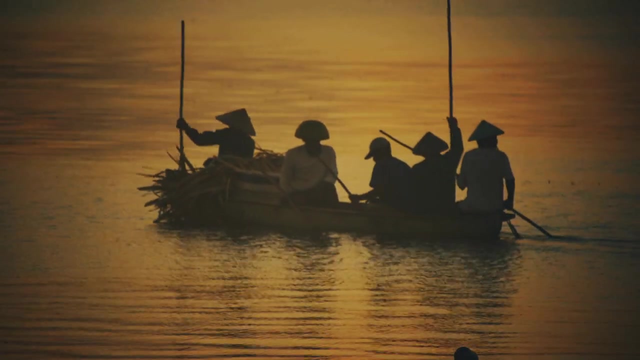 It supports the healthy functioning of the planet and the well-being of humanity. For example, marine plants produce roughly 50% of atmospheric oxygen. Coral reef-related tourism generates more than $37 billion each year. Marine fisheries and aquaculture contribute substantially to the income of more than 10% of the world's population, primarily in developing countries. 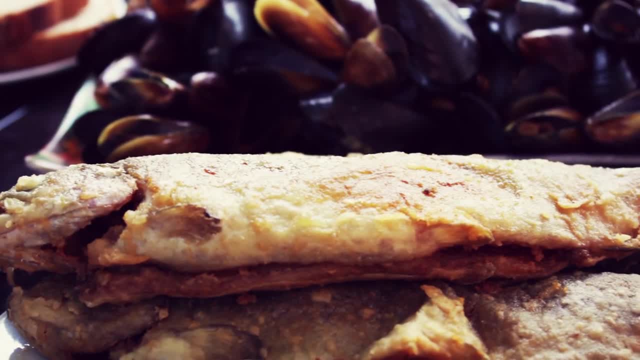 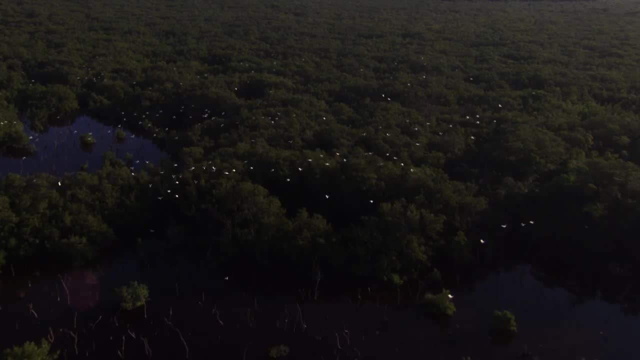 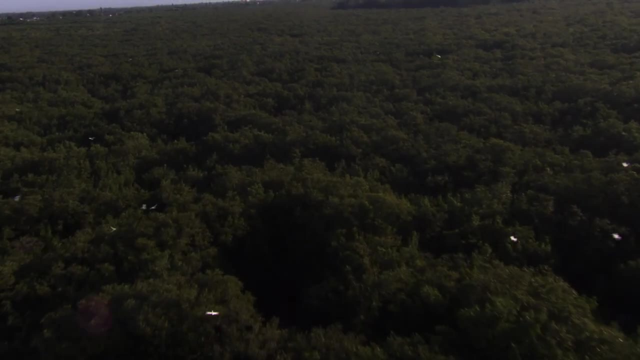 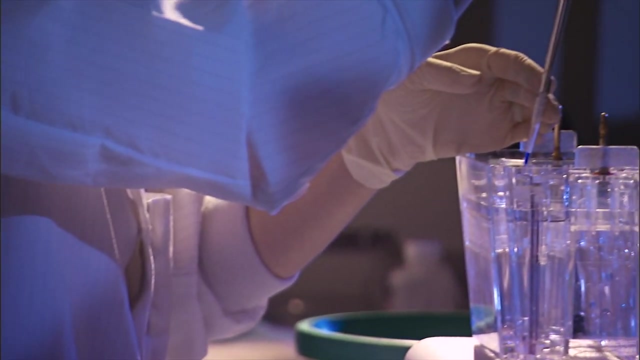 Fish provides a critical source of protein and nutrition for more than 3 billion people. Coastal ecosystems such as reefs and mangroves protect coastal communities from storm surge and extreme weather events. More than half of the nearly 5,000 patitent genes of marine organisms are being applied to medicines and human health. 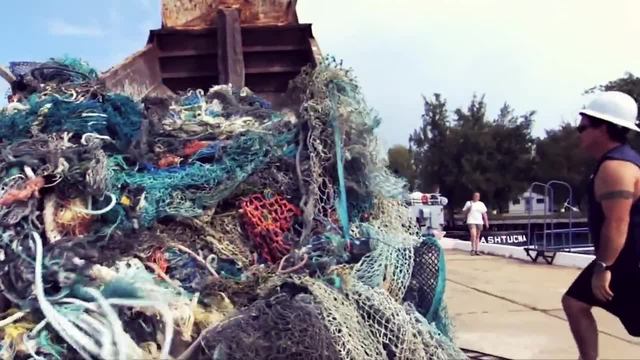 The ocean, however, is changing. It is under increasing pressure from our natural resources. It is under increasing pressure from our natural resources. It is under increasing pressure from our natural resources and sustainable fishing practices, pollution, marine debris, habitat loss, ocean acidification and climate change. 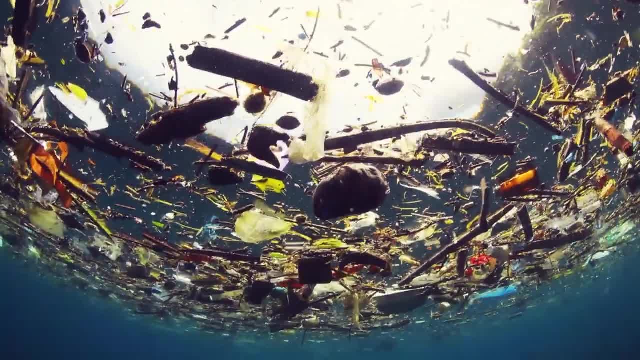 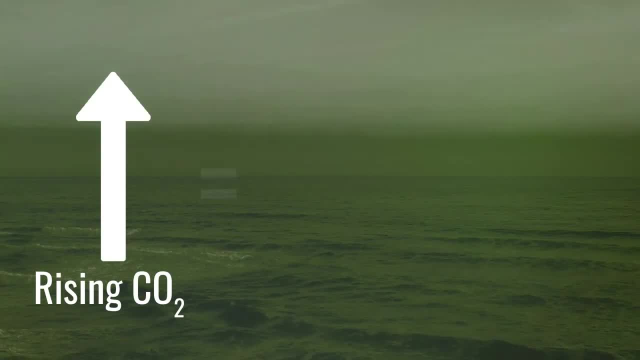 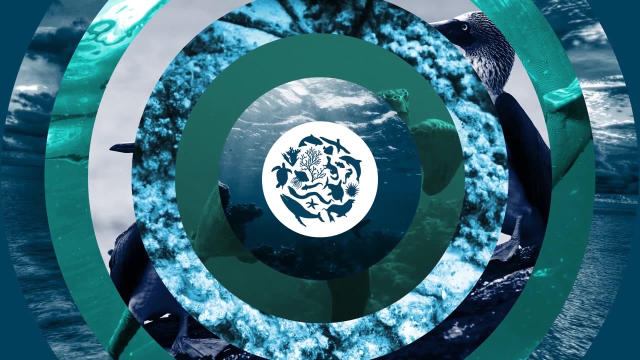 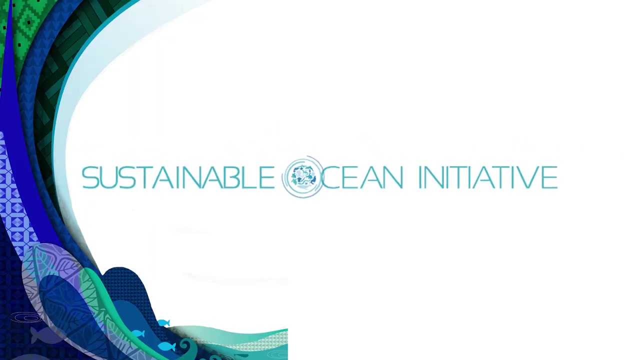 and sustainable fishing practices, pollution, marine debris, habitat loss, ocean acidification and climate change. Protecting and restoring marine biodiversity is critical to achieving the future we want—sustainable oceans. Parties to the Convention on Biological Diversity have been working together with partners around the world. 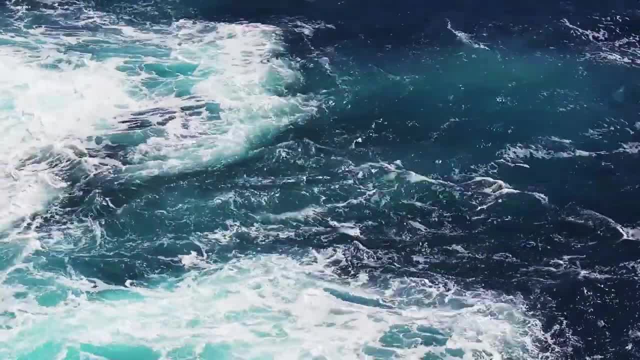 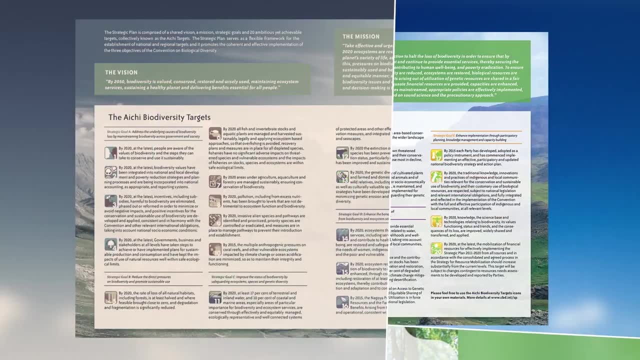 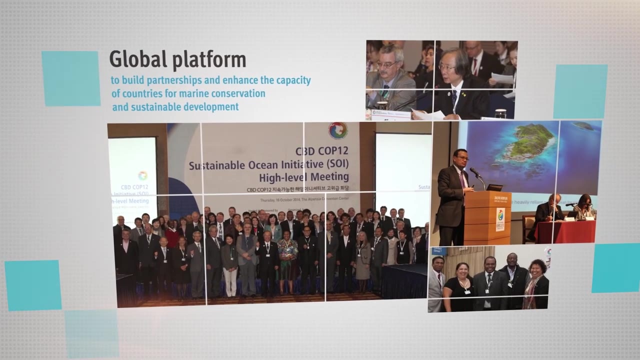 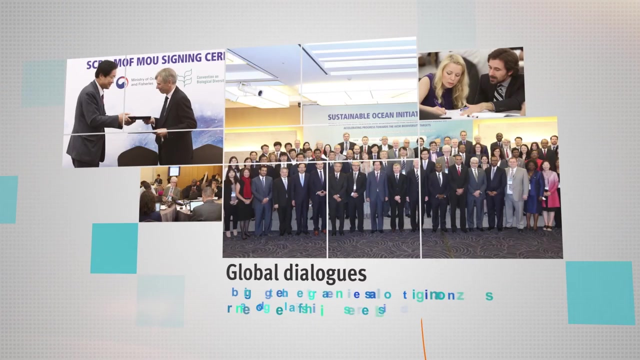 have been working together with partners around the world world to safeguard marine biodiversity through the Strategic Plan for Biodiversity 2011 through 2020 and its 20 HE biodiversity targets. Our experience and progress will contribute directly to achieving Sustainable Development Goal 14.. Now is the time to make a clear choice. Let us choose to.